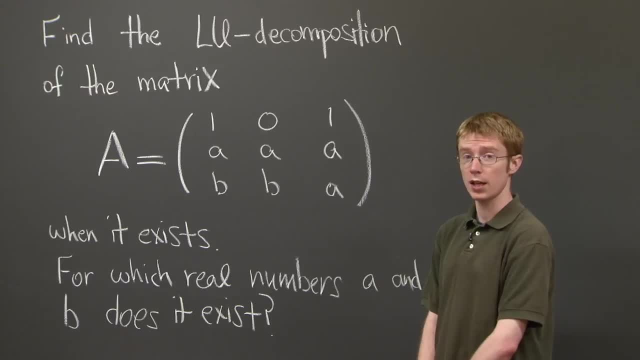 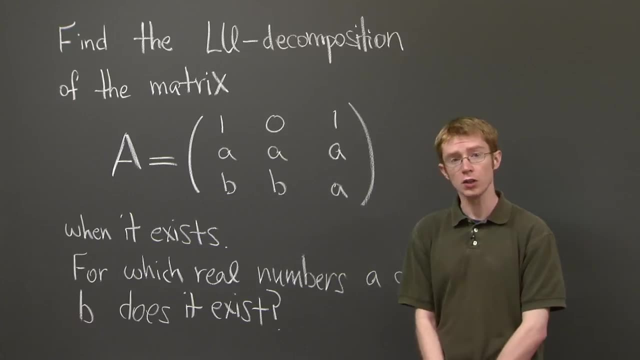 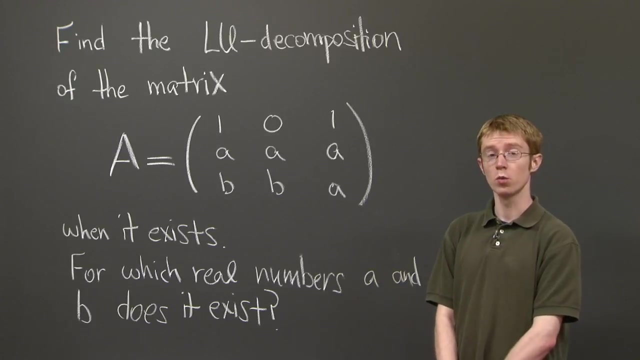 And the second part of the question asks you: for which real numbers, A and B, does the LU decomposition of this matrix- actually exist? Now you can hit pause now and I'll give you a few seconds. You can try to solve this on your own and then we'll be. 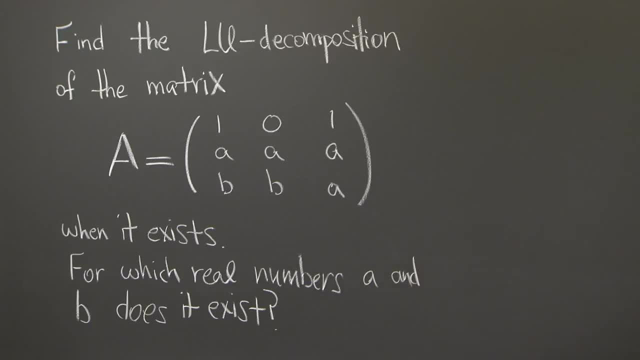 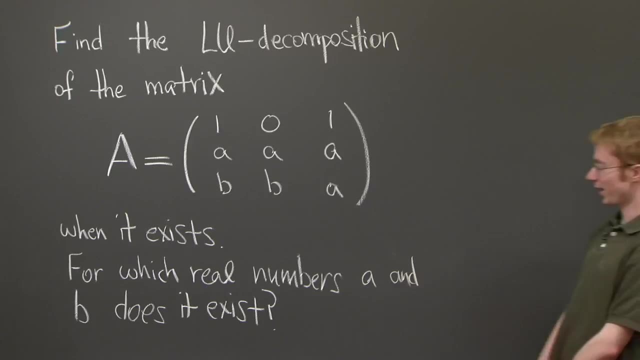 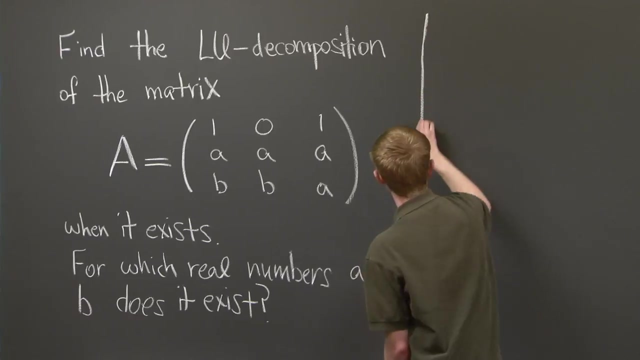 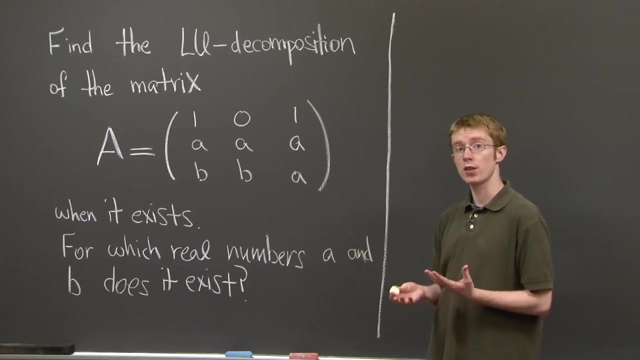 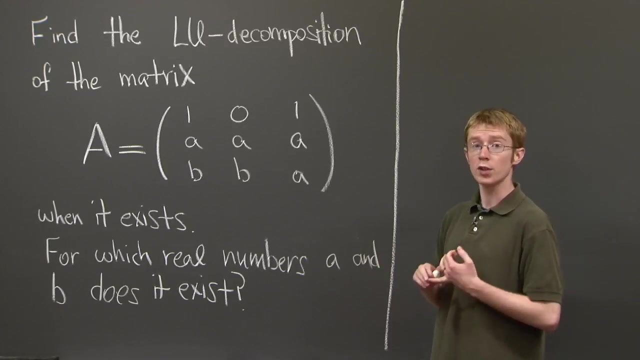 back and we can do it together. And we're back Now. what do you have to remember when doing an LU decomposition problem? Well, we do elimination in the same way that we did before in order to find U, But with With this question, we need to find L as well. 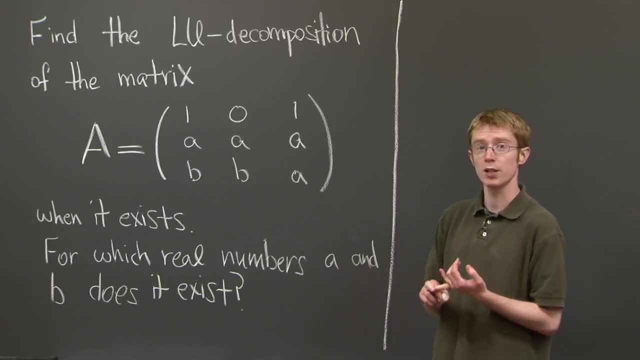 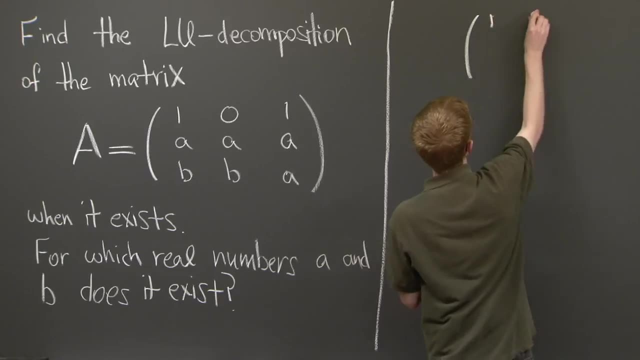 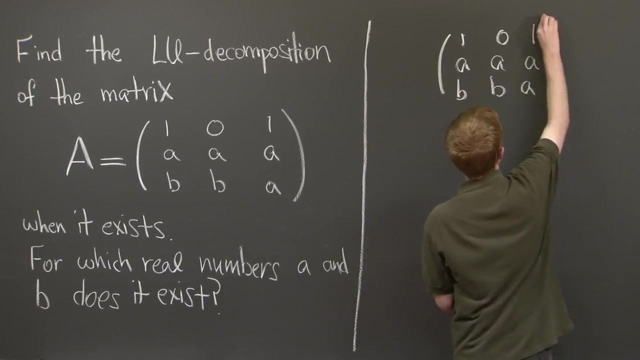 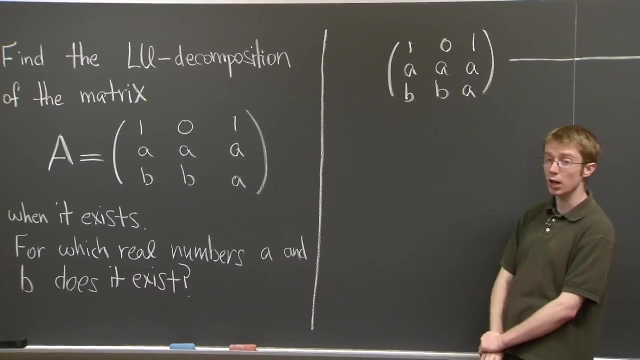 So we need to do elimination, but we also need to keep track of the elimination matrices along the way. Good, So let's do that. So let me put my matrix up here. And we want to do elimination. So which entry do we eliminate first? 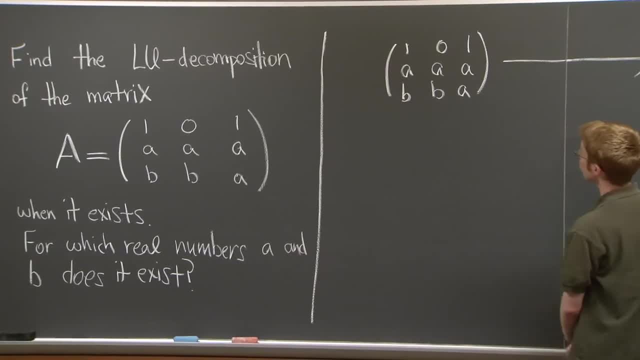 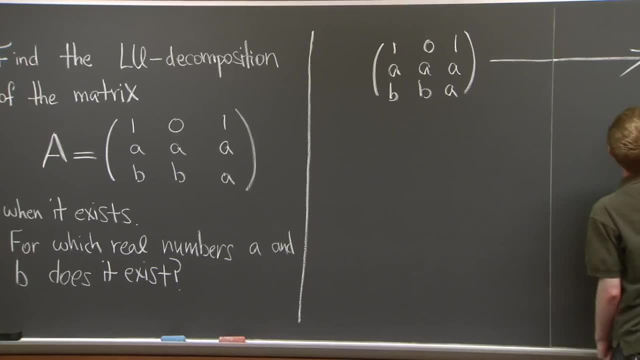 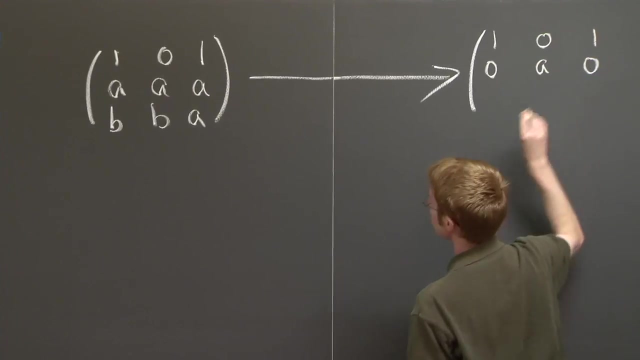 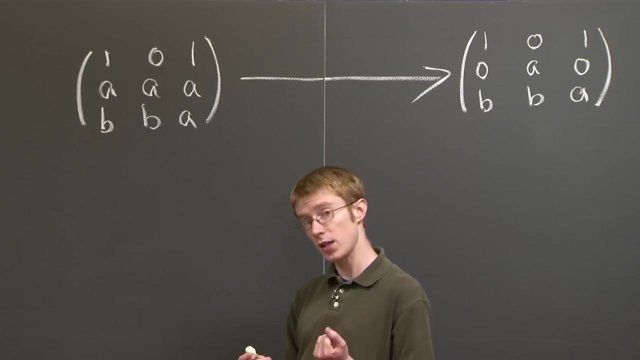 That's right. It's this 2, 1 entry. So we replace the second row by the second row minus A times the first row, And we get this OK. But we're not just doing elimination, We're finding an LU decomposition. 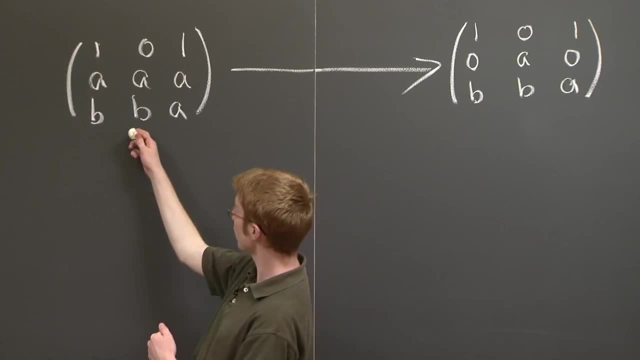 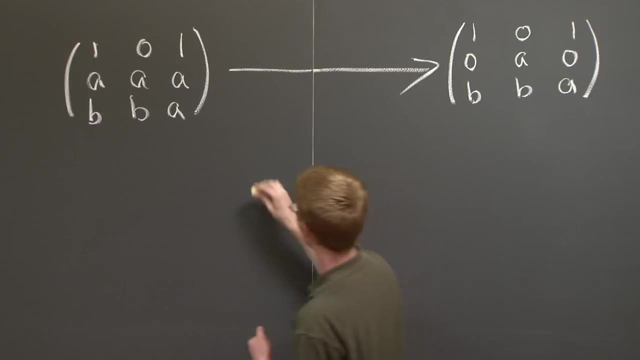 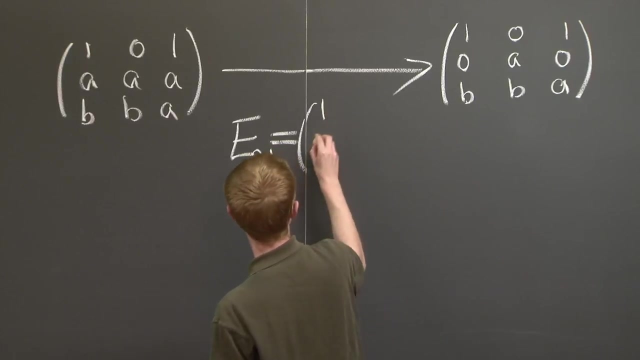 So we need to keep track of the matrix that I multiplied The elimination matrix, that I multiplied this matrix A by on the left to get this matrix. So what is that? That's this E 2, 1.. Since I eliminated the 2, 1 entry, I'll call it E 2, 1.. 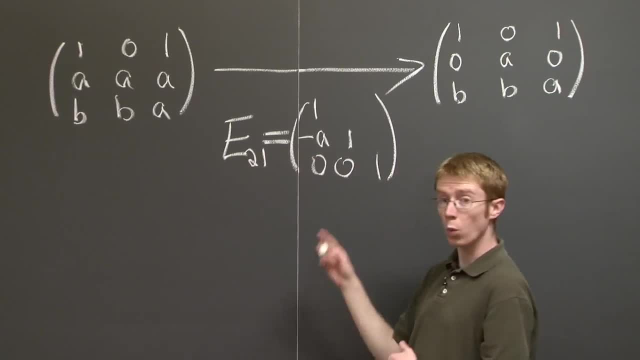 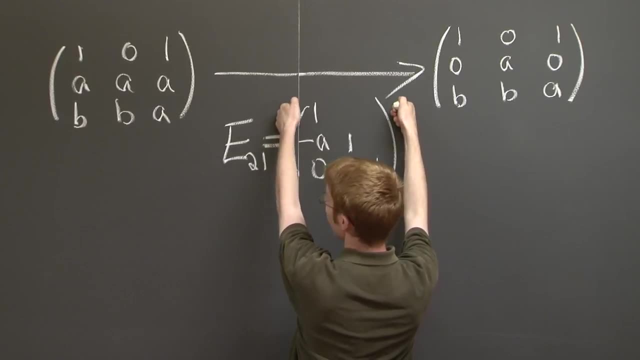 And it's this matrix. Why is it this matrix? Well, remember how multiplication on the left works. I replaced the first row by just the first row. I replaced the second row by just the first row. I replaced the second row by the second row minus A. 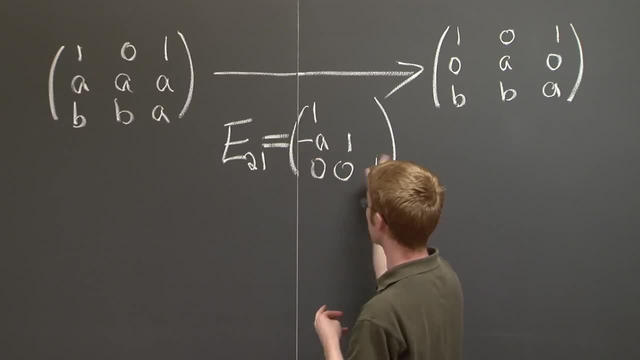 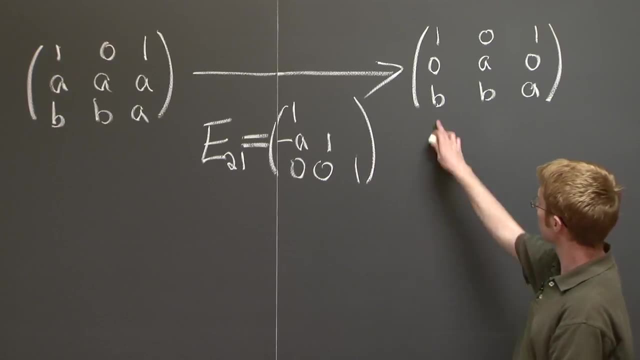 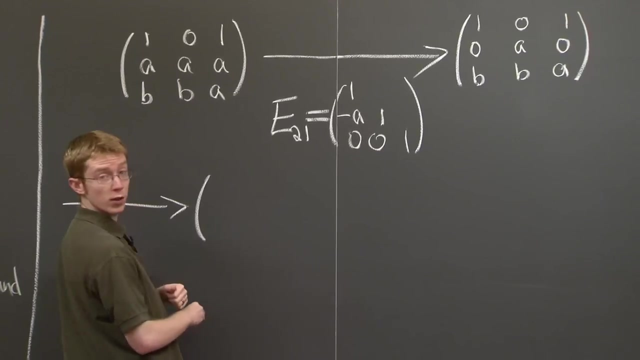 times the first row. So you can just read off from these rows which operations I did Good. Now which entry should we eliminate next? We need to eliminate this B, So we will replace the third row by the third row minus B times the first row. 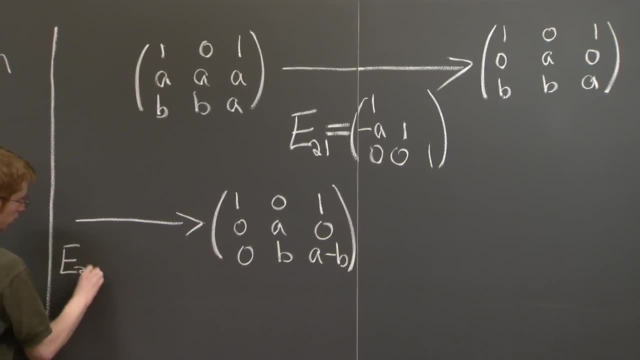 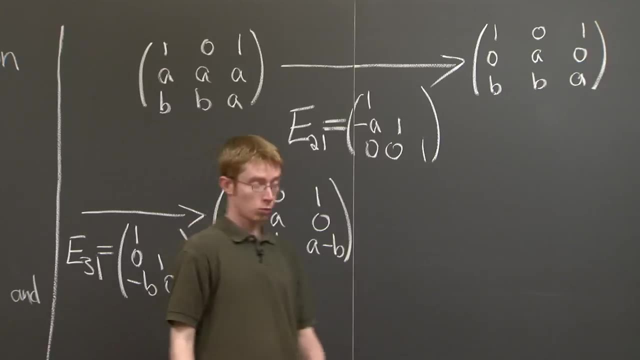 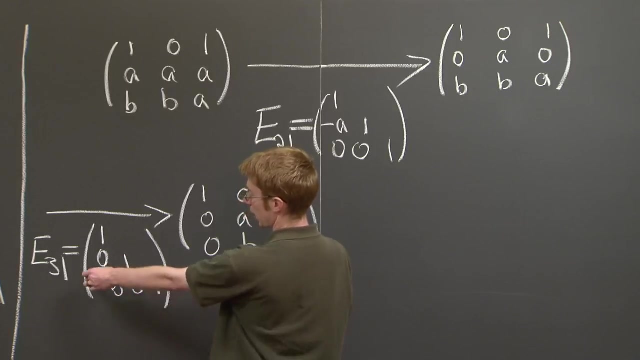 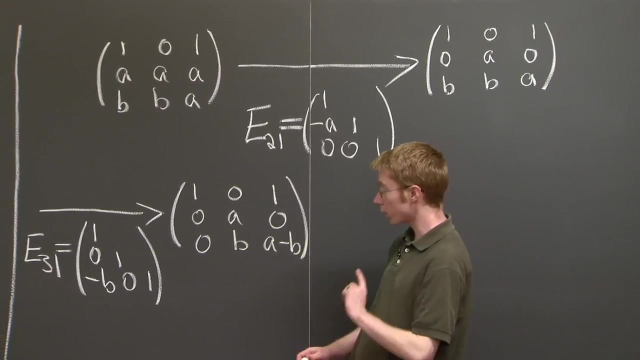 And which elimination matrix did we use? Well, note: we replaced the third row by the third row, minus B times the first row. That's exactly what you should read off this elimination matrix. Good, Now we only have one step left right. 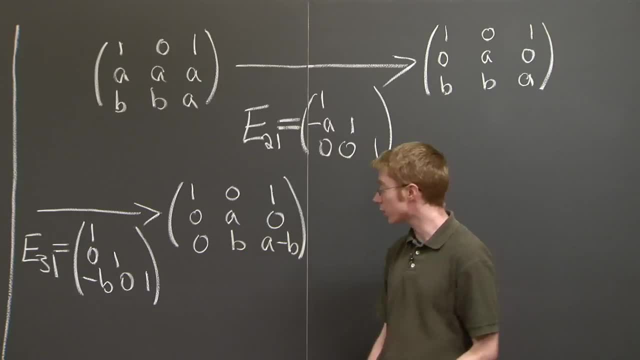 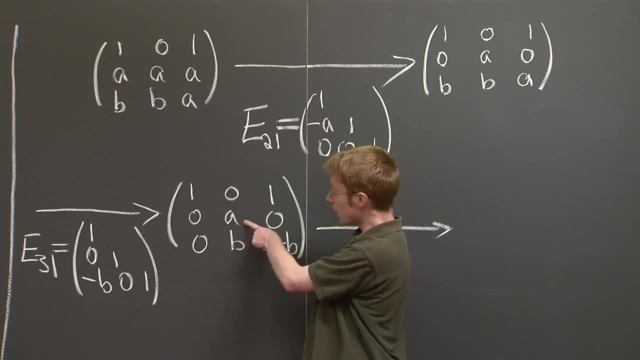 We only need to eliminate one last entry, But this one's a little tricky. So let's see. So let's be careful. In order to eliminate this B, we need A to be a pivot. In particular, we need A to be non-zero. 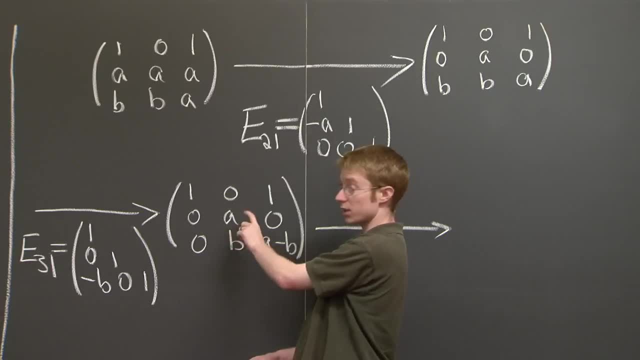 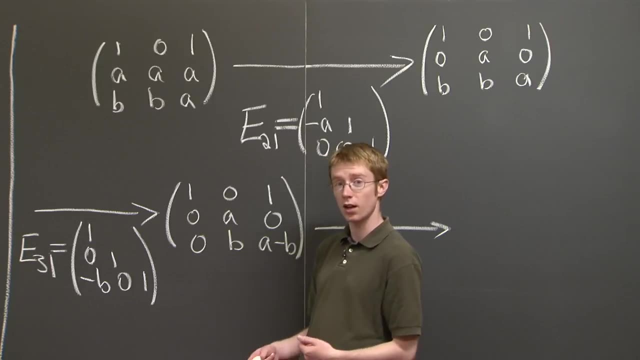 If A were 0 here, then we would have to do a row exchange, And that's no good. You can't find an LU decomposition if you have to do a row exchange in elimination, So we need to assume that A is non-zero. 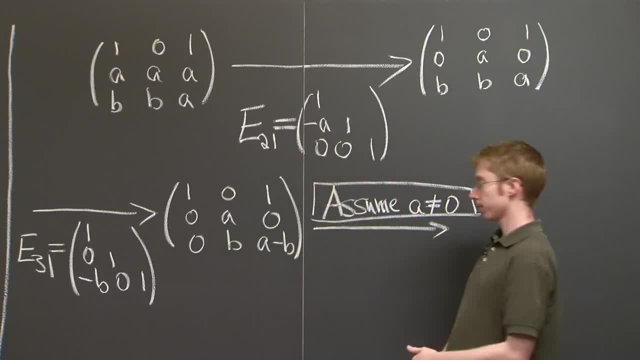 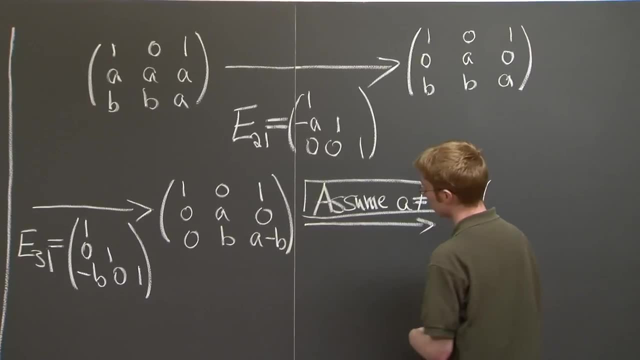 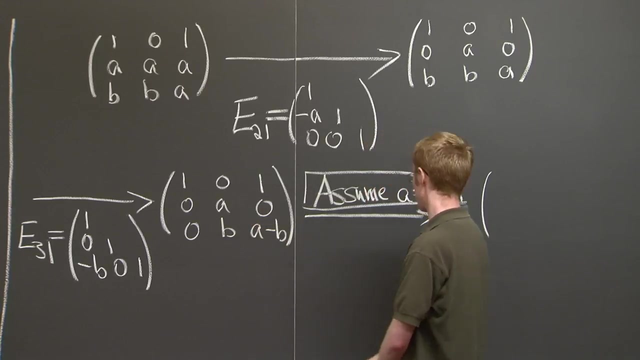 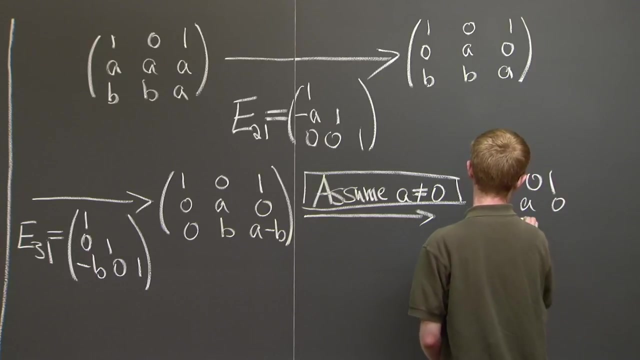 In order to keep going. OK, So let's just assume there that A is non-zero. Now what do we do? Well, we can replace the third row by the third row minus B over A times the second row, And we just get this. 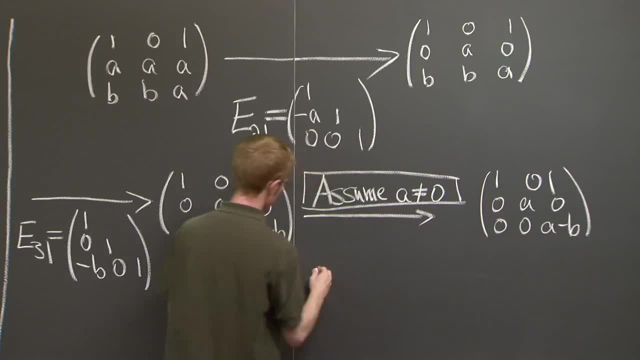 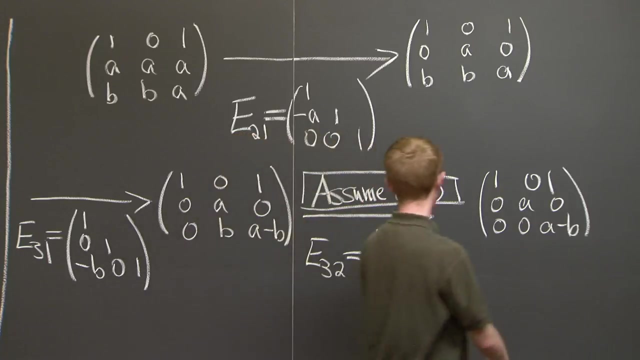 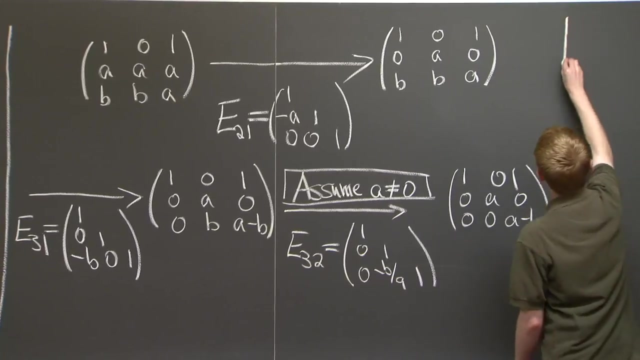 A minus B. Good, And let's write down our elimination matrix E32. now There's our elimination matrix. We replace the third row by the third row minus B over A times the second row. Good, So we found our U matrix. 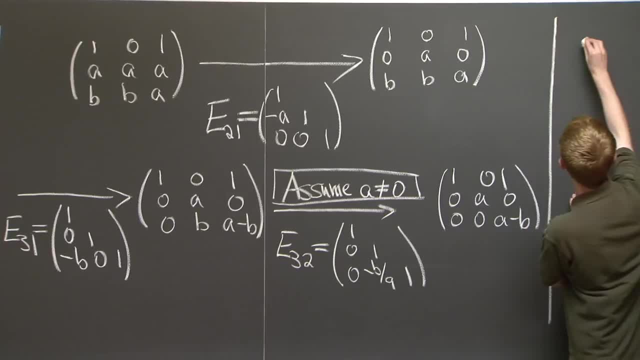 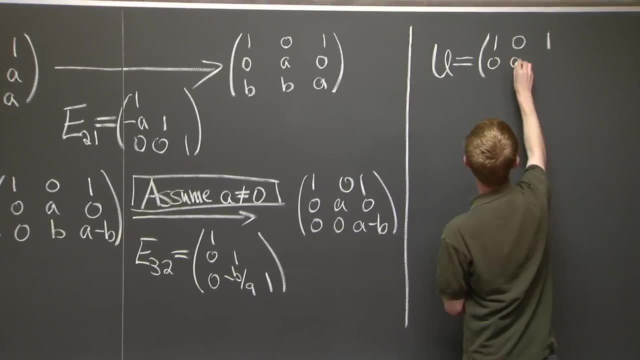 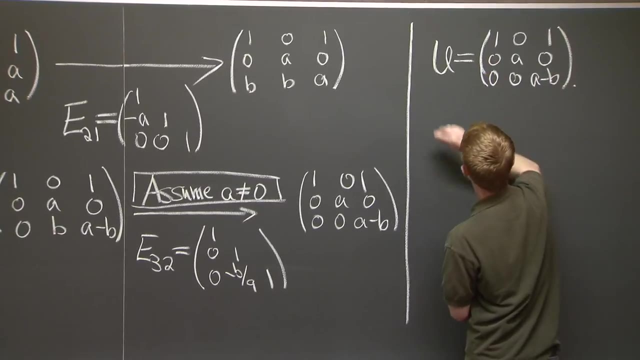 That's what elimination does. It gives us our U matrix, So let me write it up here: 1, 0, 1, 0, A. 0, 0, 0, A minus B. Good OK. 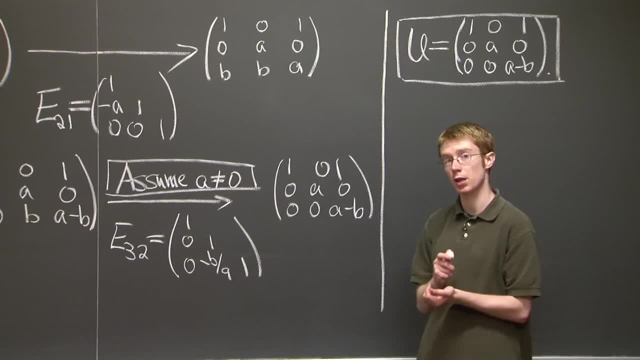 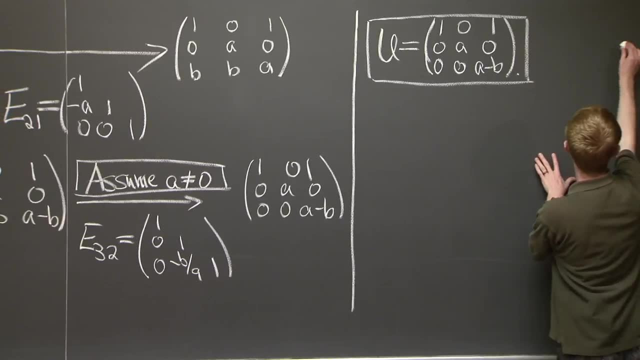 Now we have to find our L matrix And we need to use these elimination matrices that we've been recording along the way in order to do that. OK, So remember that we started with A and we got U, And how did we do that? 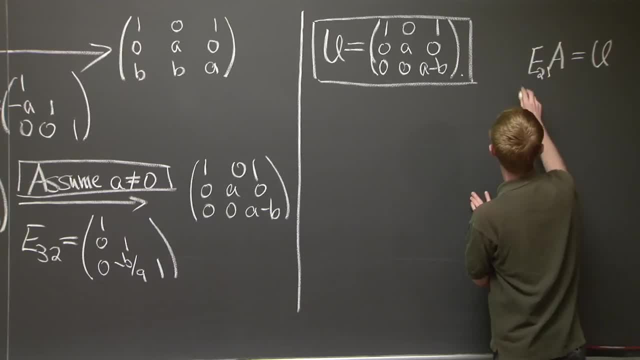 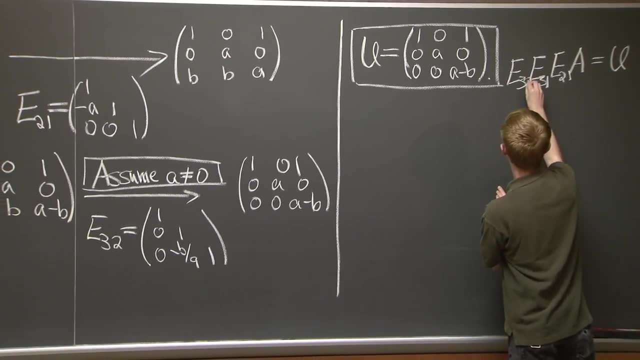 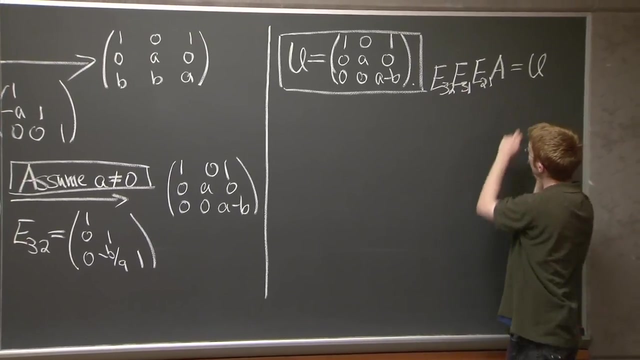 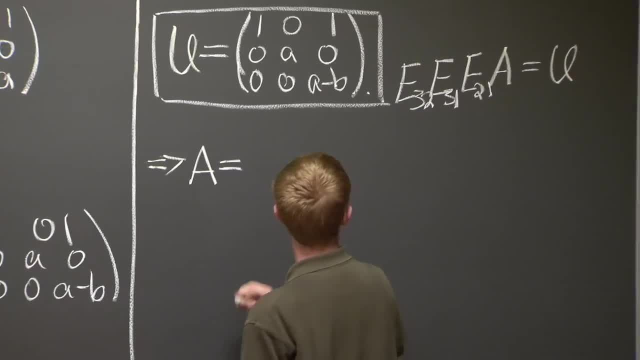 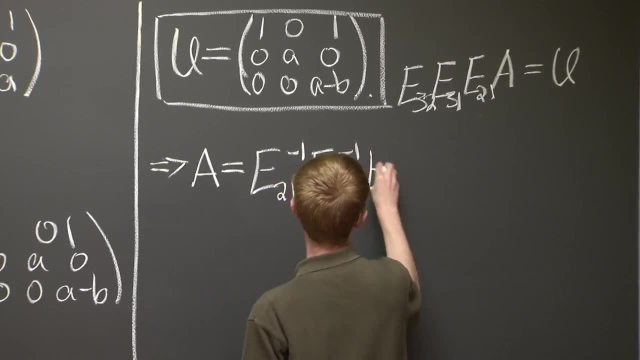 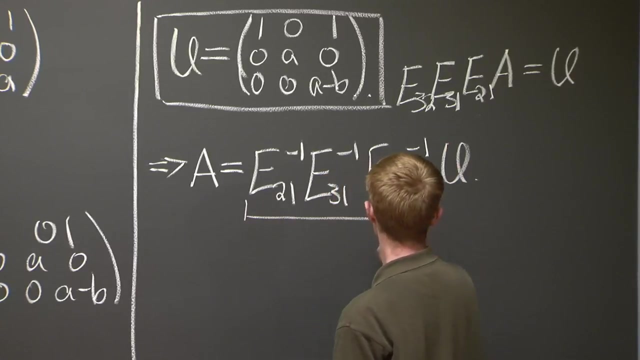 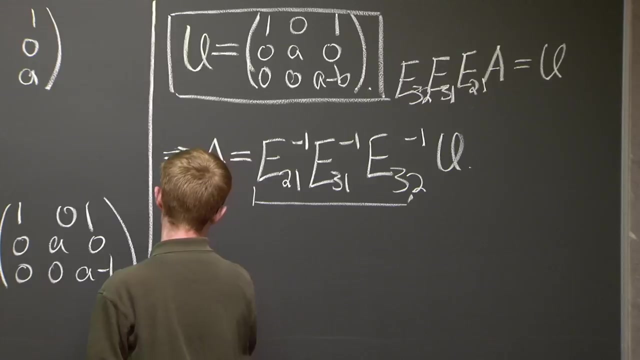 And E32. And E32.. So what do we have? We have A equals E21, inverse E31, inverse E32, inverse times U, And this is our L, this product of these three matrices. Good, So let's compute it now. 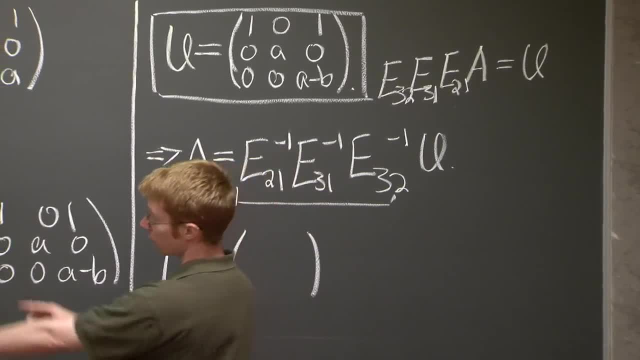 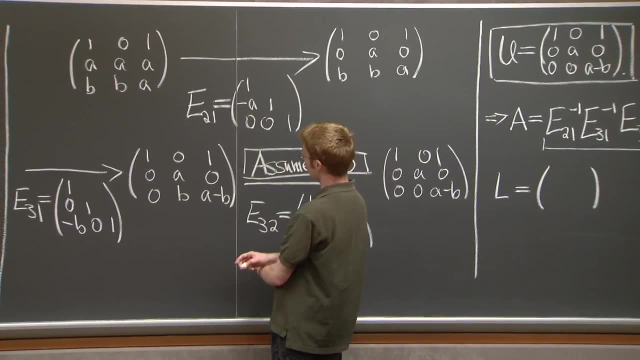 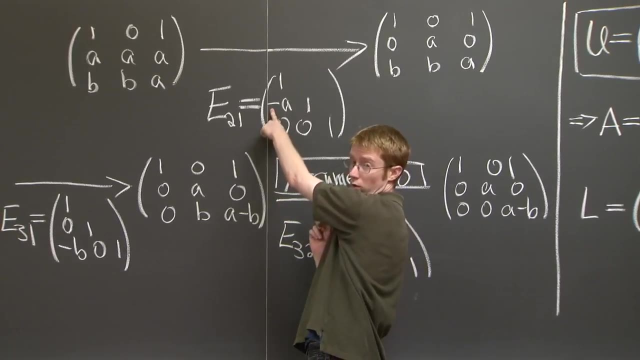 Right, So L is the product of three matrices. I need to get them by going back and looking at these three elimination matrices and taking their inverses. Well, the nice thing about taking an inverse of an elementary matrix like this is we just make a minus a plus or a plus a minus. 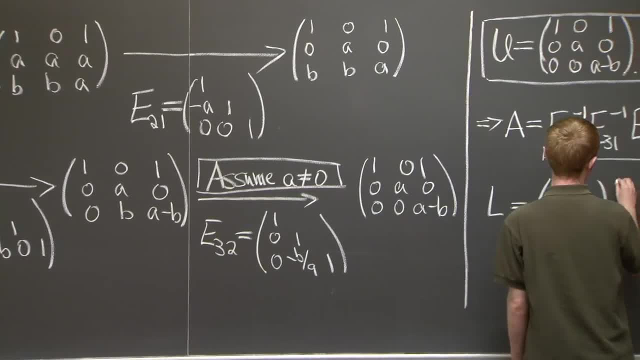 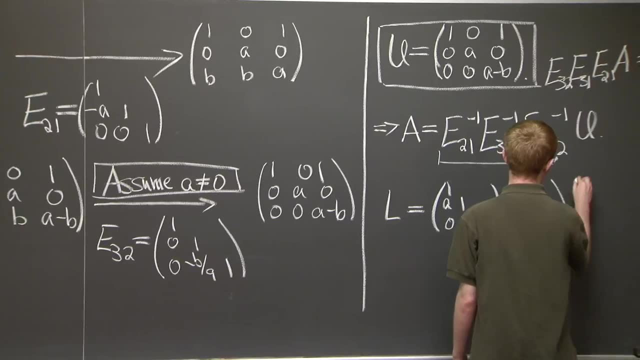 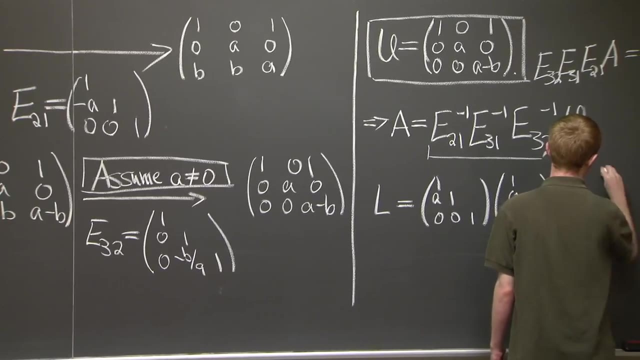 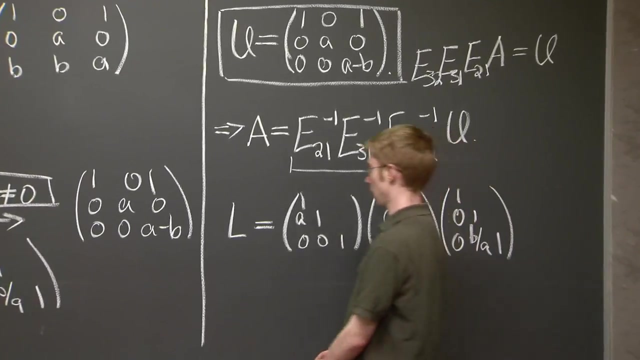 So that's easy enough. We just change the off-diagonal entries, We just change their signs. You can check that that does what we wanted it to, gives us the inverse Good. And the last comment is that multiplying these three matrices is really easy in this order. 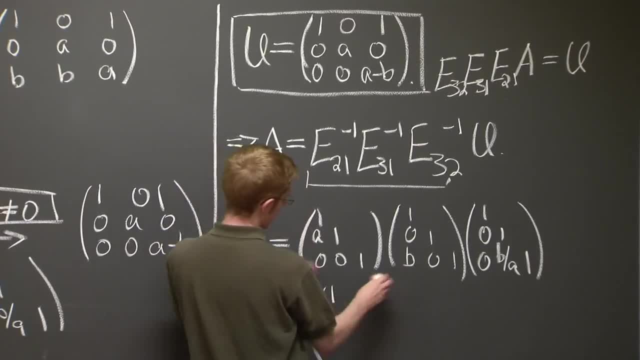 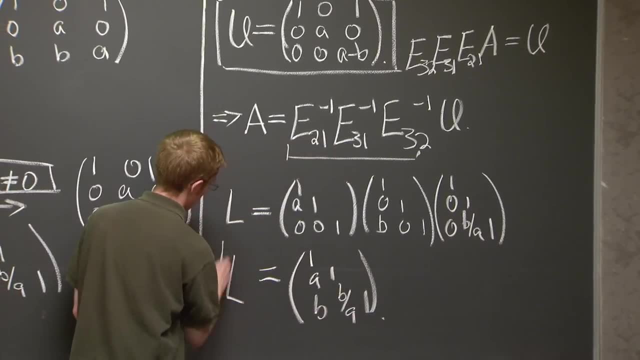 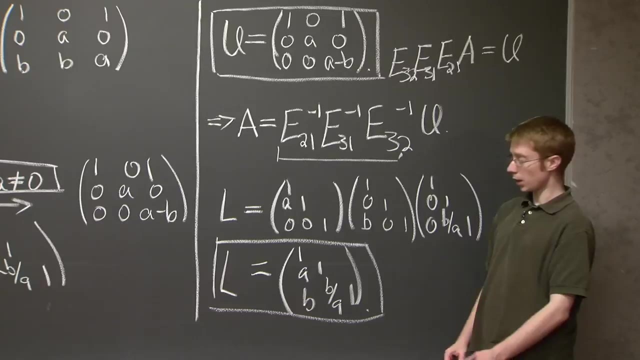 Turns out. all you do is you just plop these entries right in: 1, 1.. Good, So this is our L matrix. So now we have our U matrix and our L matrix And we're done with the first part of the question. 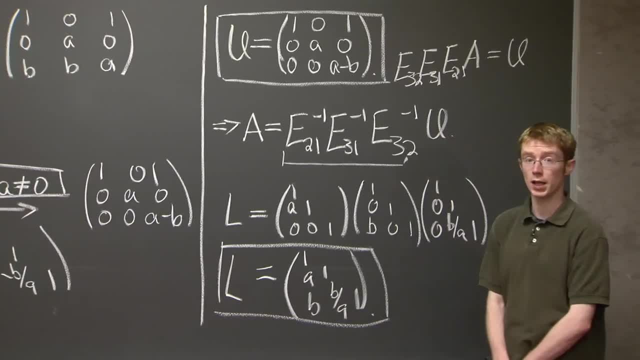 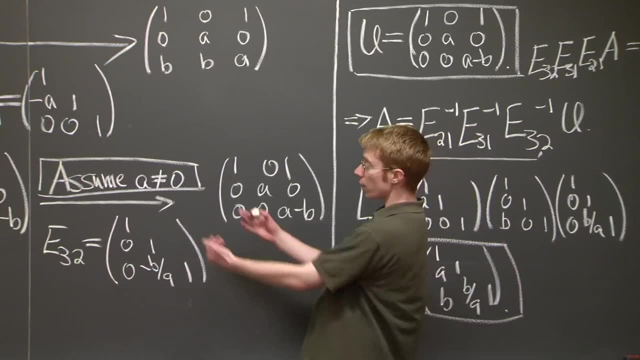 The second part asks us for which real numbers, A and B, does this decomposition exist? Now let's go back and remember that at one point we had to assume that A was non-zero. That was the only assumption we had to make to get this decomposition.